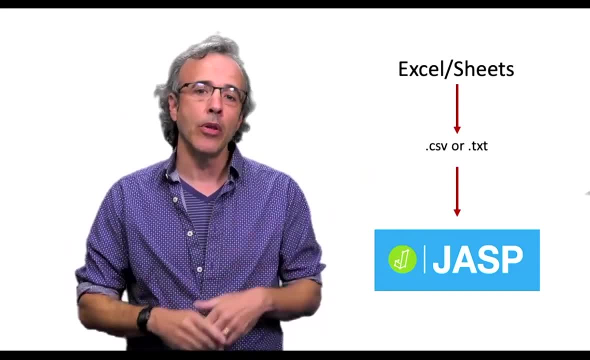 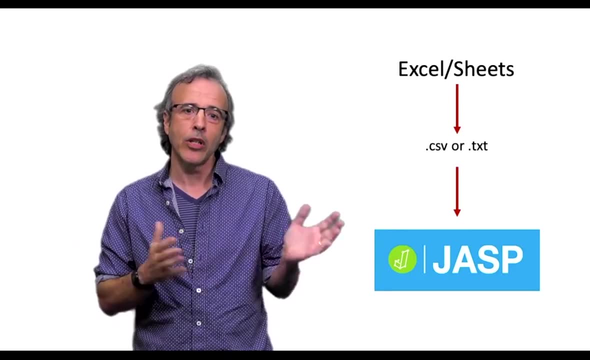 walk slowly, then people, And so one thing you've got to figure out is what kind of data you're collecting. We're going to talk about two different kinds of data: dichotomous data or continuous data. So if you're collecting- 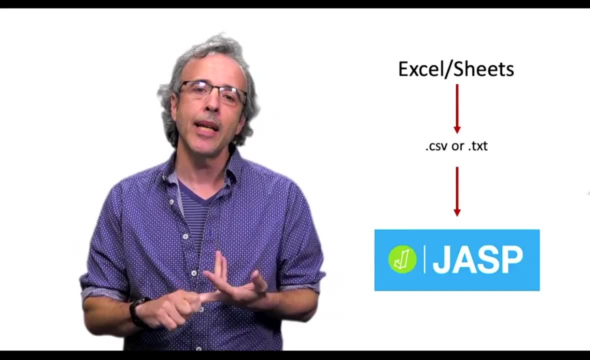 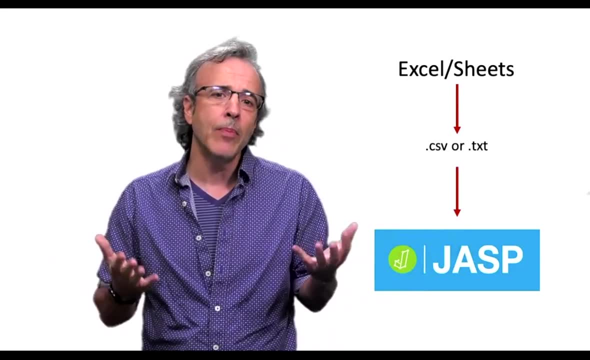 dichotomous data. what you're doing is collecting an outcome that either does occur or doesn't occur. So, for example, you might want to know if people who are using a cell phone are more likely to sort of be blindly tumbling around the world. So if you're collecting dichotomous data, 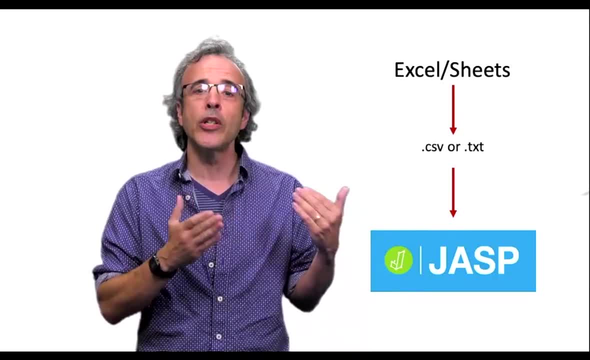 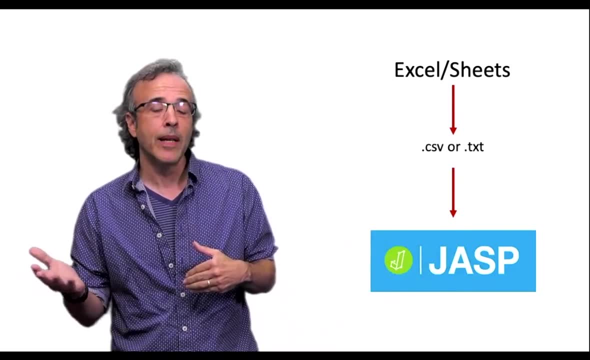 you're going to want to know if people who are using a cell phone are more likely to sort of be blindly tumbling around the world and getting into a collision. So what you're coding is: yes, a person got into a collision or no, they didn't get into a collision. And then you're noting: 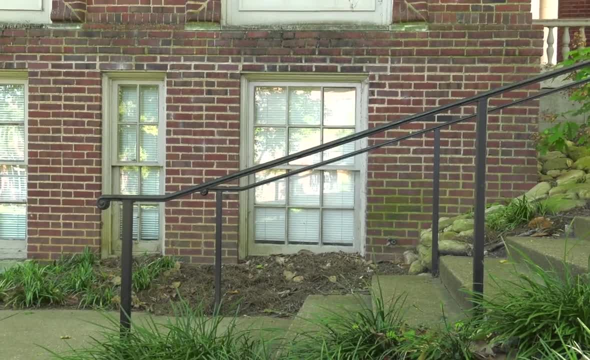 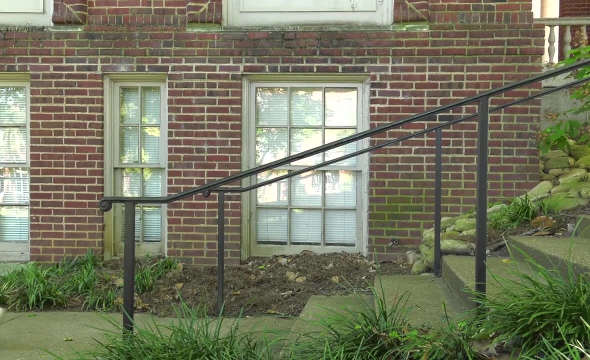 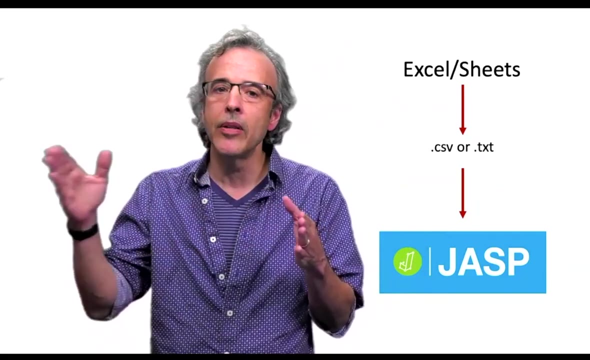 whether or not they were using a cell phone. Alternatively, you might want to know if using a cell phone makes people walk more slowly, say when they're going down the stairs. So in this case, your dependent variable is continuous. It can take any of a number of values going from: 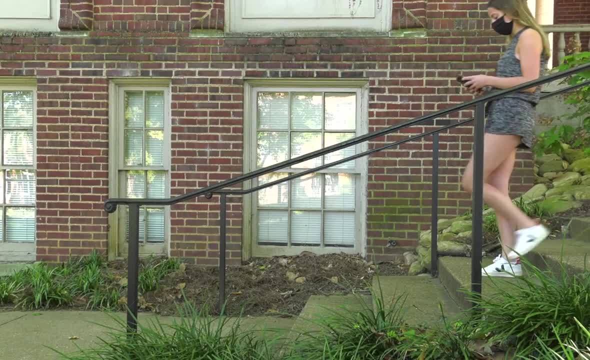 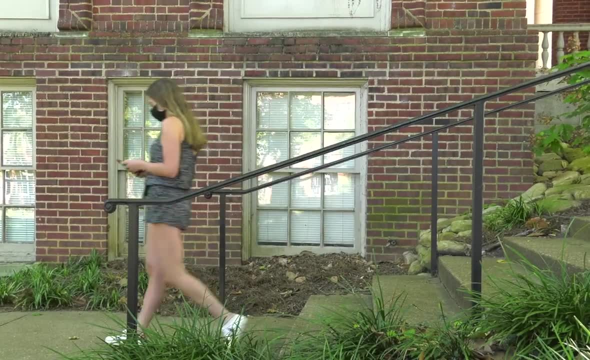 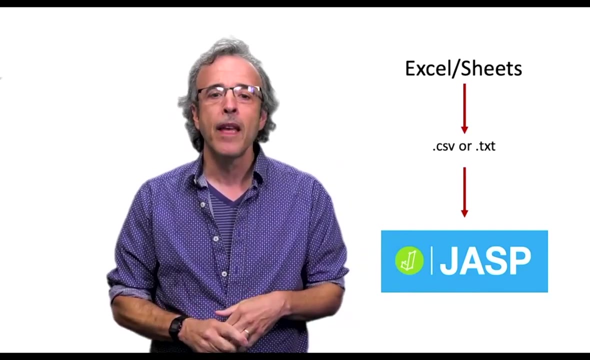 low to high in order. So someone might walk slowly taking eight seconds, they might go a little faster- seven, really fast- six or five seconds, And so those are two kinds of data that we're going to sort of explore using JASP. The other thing you have to realize is that in this particular 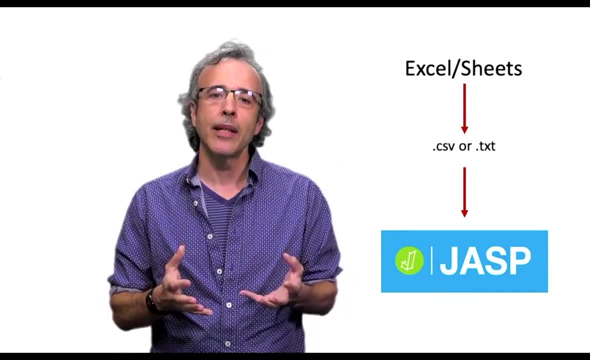 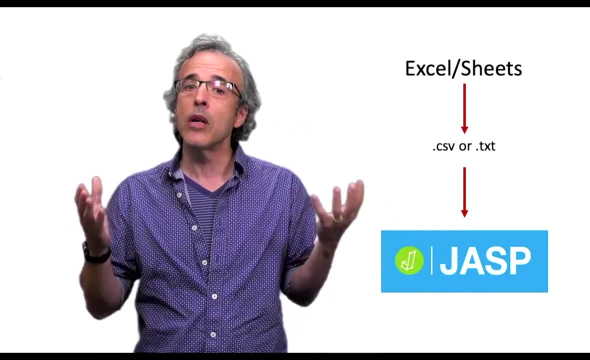 experiment. we've got a between subjects design. we're going to be observing some people who are using a cell phone and then other people who are using a cell phone and then other people who are using a cell phone, And so that between subjects design affects how we set up data. So the first: 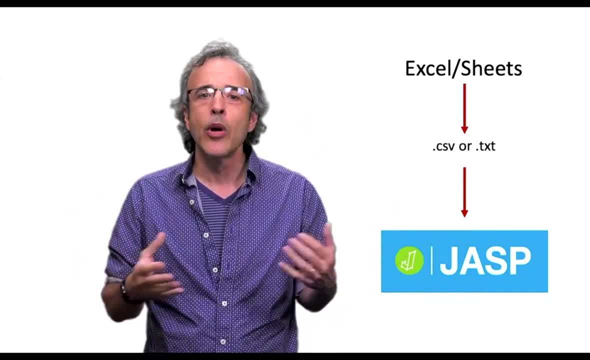 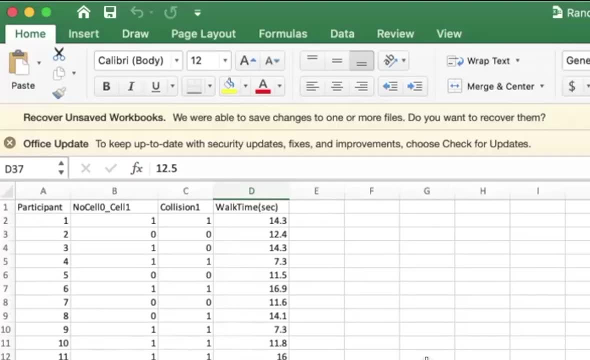 step is to imagine you've collected your data And now we're going to take a look at how you set up those data in Excel or Sheets. Okay, so what we're looking at here is some example data. This is a data file that has basically random data that I made up in it And the first thing you notice about 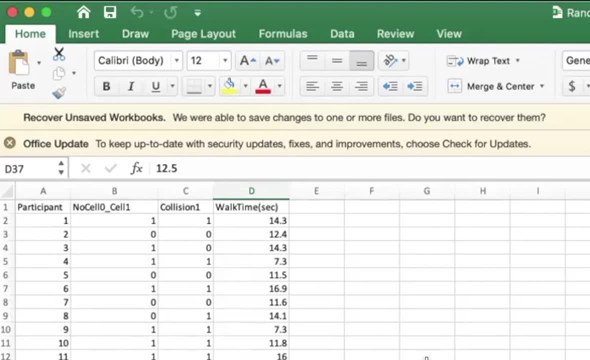 it is that it's organized into a series of columns And most of the columns name a variable. So, for example, column B here is going to specify no cell, in which case there's going to be a zero in the column, or cell phone a one in the column. Column C: here is going to be collision one zero, it's a. 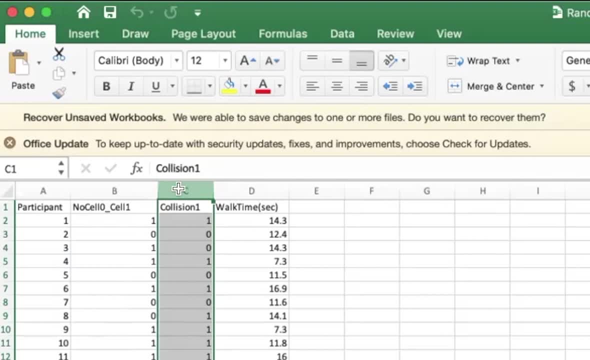 dichotomous variable. One: if the person got in a collision, zero, if the person did not get in the collision, Column D here is going to be a continuous variable, And so this would be the kind of column you'd enter if you were measuring, say, how fast someone's walking when they were walking down the stairs. So 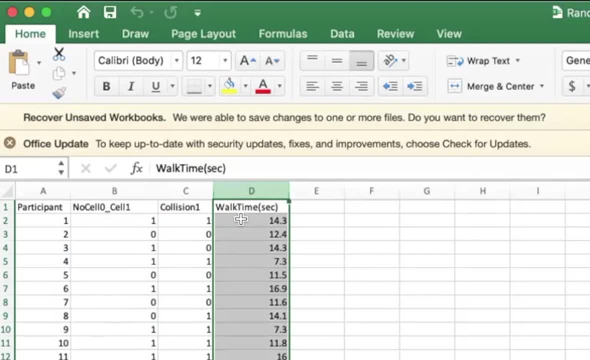 we've got walking time in seconds in column D. The first thing to really think about in terms of the organization of this spreadsheet is that every column is a variable and every row, in this case, is a participant. So, starting with row two, here we've got participant one, then participant two, three, four, five and so on going down the rows. 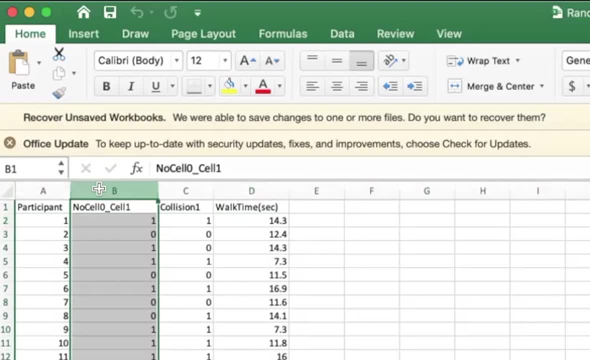 A couple of notes here. Number one: it's often nice to name your variables in the first row of your spreadsheet, So you want to do that And also to name your variables in a way that's kind of informative. I like to put a lot of information in my variables. 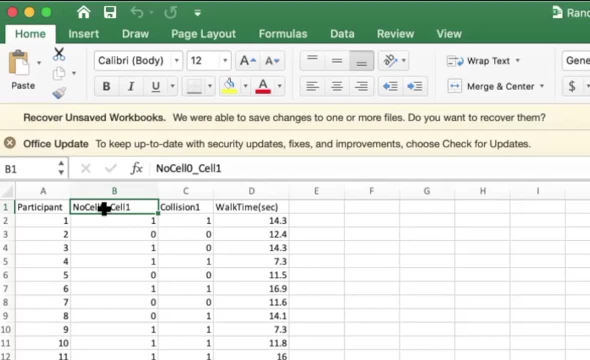 So this variable name which is going to show up in JASP is no cell, zero cell one, And so that tells us what the variable is, and it also tells us a little bit about how the variables coded. So zero means this participant was not using their cell phone, one means they were using their cell phone. 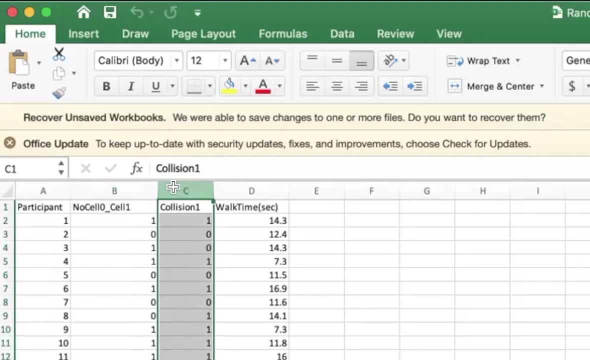 And then we've got collision one here. So collision is coded as a one, and then we can assume that a zero means no collision. And then walk time. that's pretty straightforward, It's the walking time. It's the walking time. 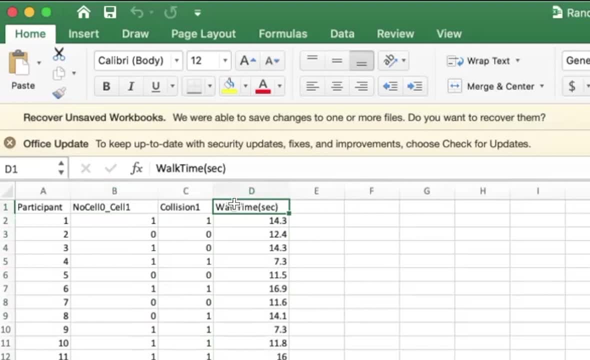 The walking time and I put those sort of that- it's in seconds- in the variable name. Okay, so that's the organization of your data file. Take a close look and try to match your data to something kind of like this: One key thing to realize is that when you save your data to use in JASP, you have to save it out as a text file or a CSV file. 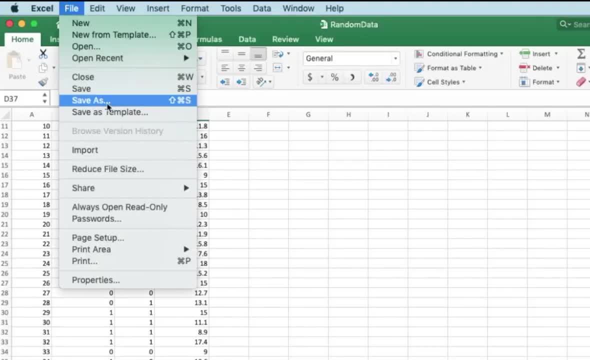 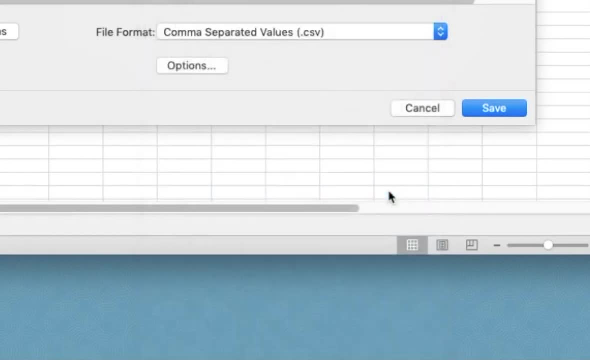 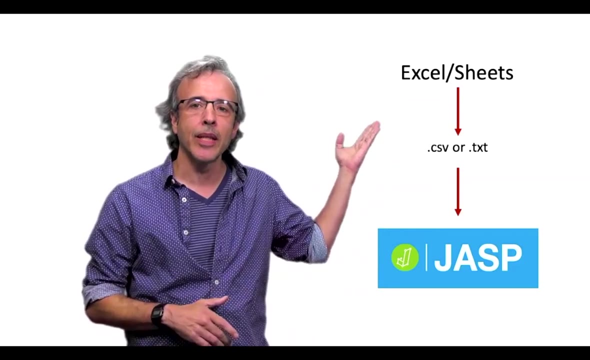 JASP won't open an Excel file. Do a save as and then just select CSV here, And so it will save as a CSV and I'll replace that one because I already saved it. Okay, so now we've saved our data out from Excel as a CSV. Next we're going to go into JASP to analyze the data. So let's take a look. 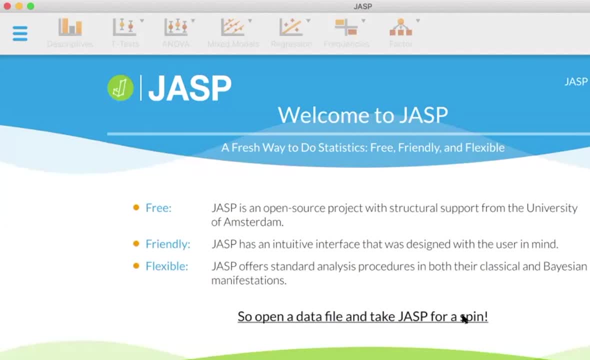 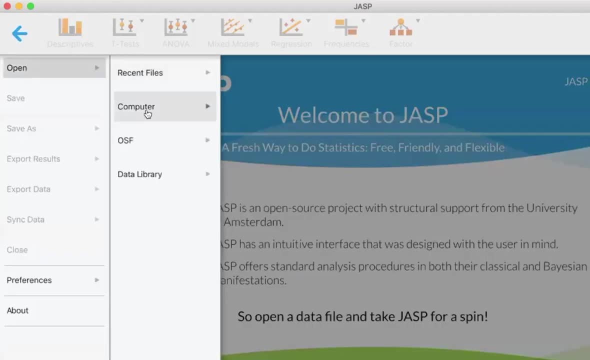 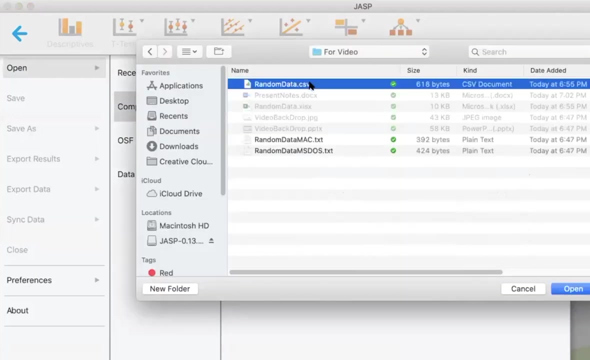 So here is the start screen for JASP, What you do to open up your data. Let's go to that little hamburger there, Go open, and usually using computer browse is the easiest way to go- And there's our random data, our CSV file. 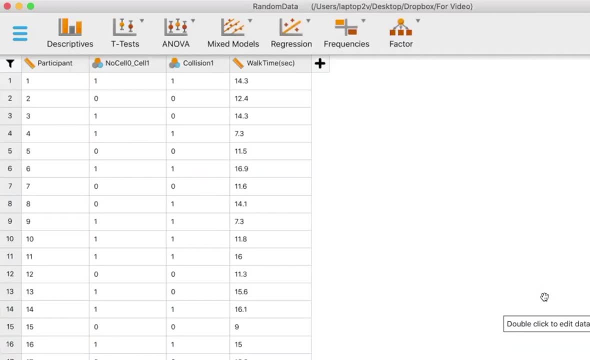 And so it opens up in JASP. There it is. So let's do two analyses. We'll do our analysis of the dichotomous variable- whether or not a person got into a collision, And then we'll also do an analysis of our continuous variable: how long it took them to walk down those stairs when they're using their cell versus not using their cell. 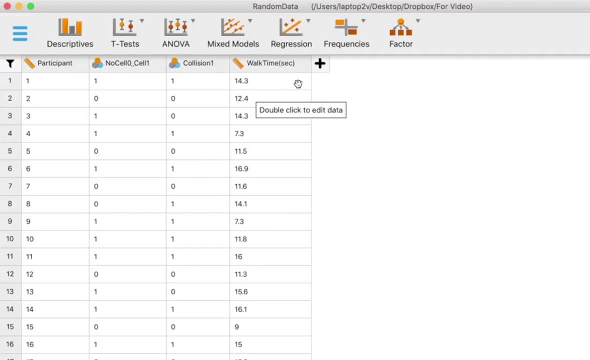 So let's start with the dichotomous variable. the way you analyze that is, you'll use a Chi Square test. That test assesses the degree to which the frequencies you've observed in a table relating your independent variable, and this is in this case cell versus no-cell. 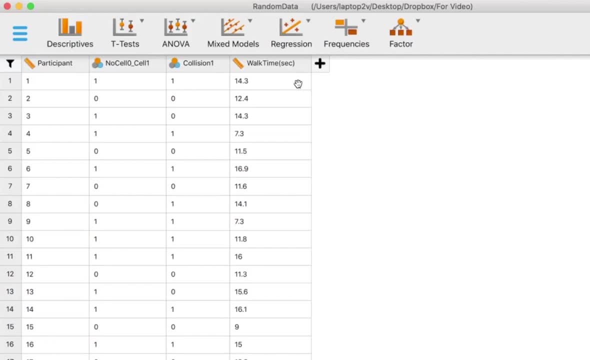 and your dependent variable and in this case your component cell case collision versus no collision. it tests the degree to which those two variables are basically independent of each other. If they're independent of each other, there's no relationship. but if 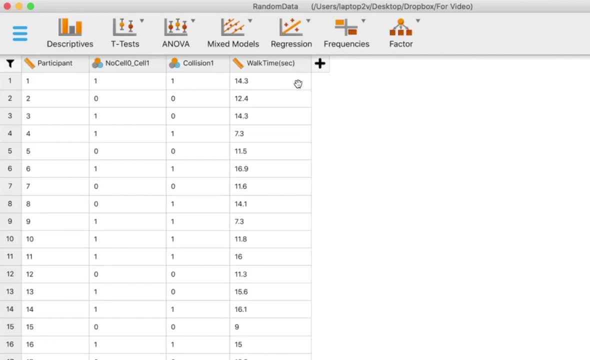 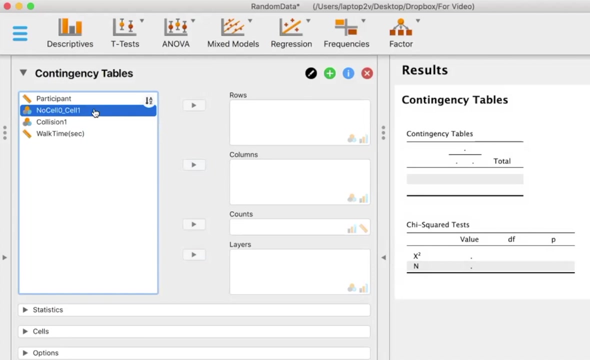 they're dependent. then there is a relationship and there may be a different rate of collisions for the cell condition and no cell condition. So the way you find that out is you go to frequencies, go to contingency tables and you want to take your variables. Remember we have no cell. 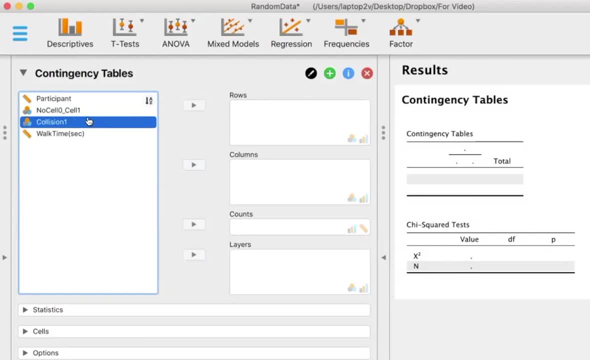 cell here and then our dichotomous variable collision, no collision, and put them in the rows and columns of a two-by-two contingency table. JASP automatically does a chi-square based on entering those two variables into your contingency table and that chi-square is output on the bottom. 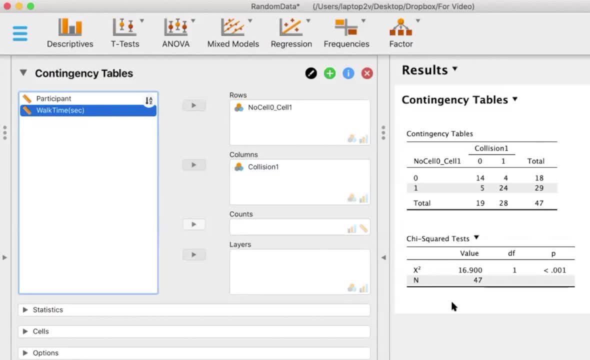 underneath the contingency table, So you can see it right here. What you've got is the result of the two-by-two contingency table, and that's the result of the two-by-two contingency table and that's the results of the chi-square test. And so let's take a look at this contingency. 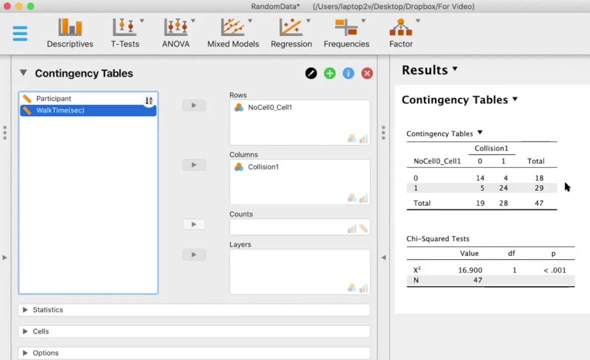 table and the chi-square test. First of all, the contingency table has two rows. In this case, row one is our participants who did not use a cell phone, and the second row, cell one, is our participants who used a cell phone. and then the columns on the table are whether or not. 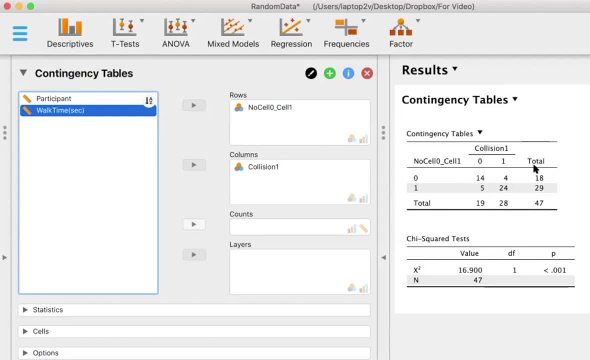 they got into a collision. So you can see, here we've got a two-by-two contingency table and we've got a total of 18 participants who were not using their cell, 29 who were using their cell phone, and out of those 18, 4 who were not using their cell phone got into a collision and 24 out. 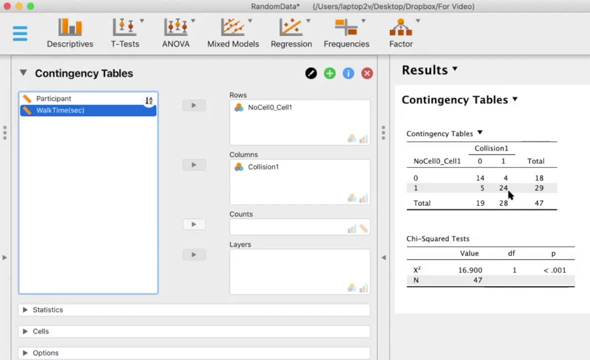 of the 29 who were using their cell phone were using their collision. 24 out of 29 subjects who were using their cell phone got into a collision, And so there's a big difference in proportions here in terms of who got into a collision. 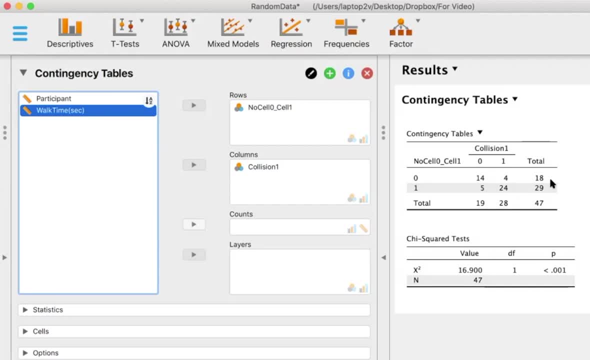 Depending on whether or not they're using your cell phone, And that's sort of what the chi-square test assesses. So our results down here are associated with a p-value and a chi-square value. The p-value here represents the probability that if you did this experiment over and over, 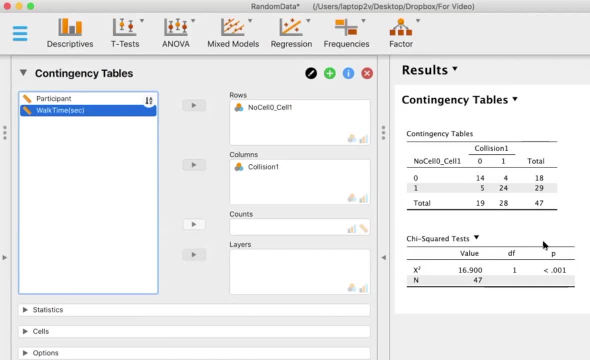 again with the same number of subjects, the same population of subjects, and there were actually nothing there that you'd observe a test value this big. So again, what that p-value represents. if you did the experiment over and over again and there were nothing there, there was, you know. your hypothesis were basically: 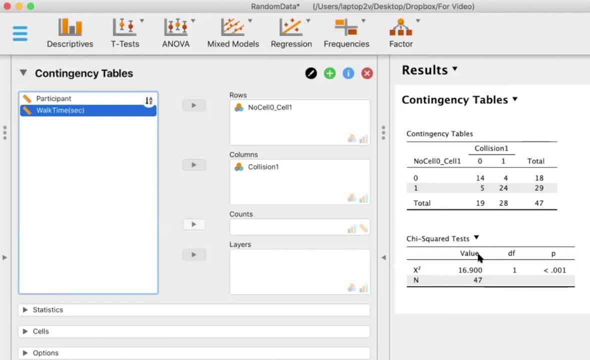 more or less wrong. The probability you get a test value that big in this case is really small, And so that means we can have some confidence that there's a real difference in the proportions of people who get into collisions when they are in our system, And so that's a big difference. 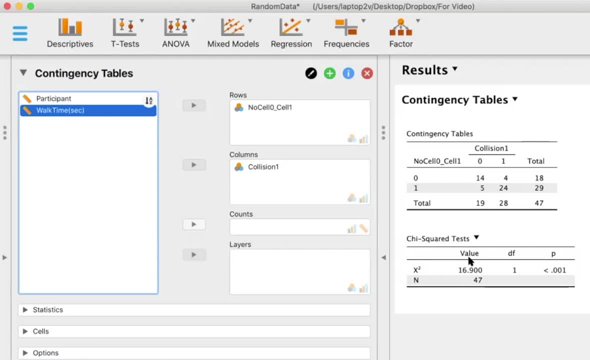 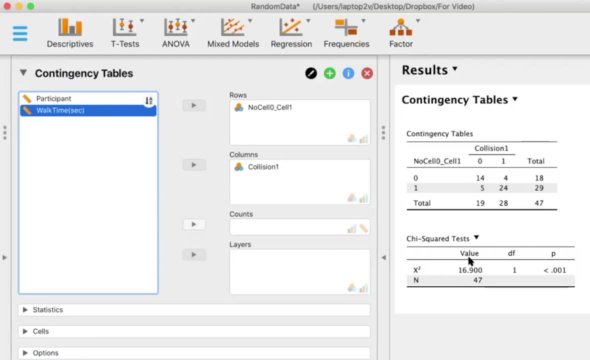 data. Let's now look at what would happen if you collected continuous data. Okay, and we're going to do a t-test to do the significance test on the continuous data. So let's close down our contingency tables and now go to t-tests up here in JASP And we're going to use 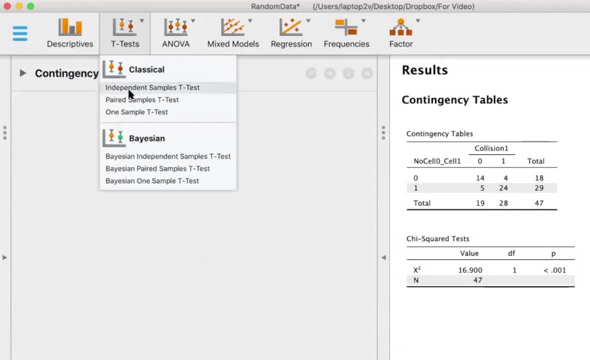 classical t-tests and we're going to use independent samples t-tests. So what that kind of test allows you to do is compare two different groups of things or people, And that's good for our between subjects experiment, because some participants were in one condition other. 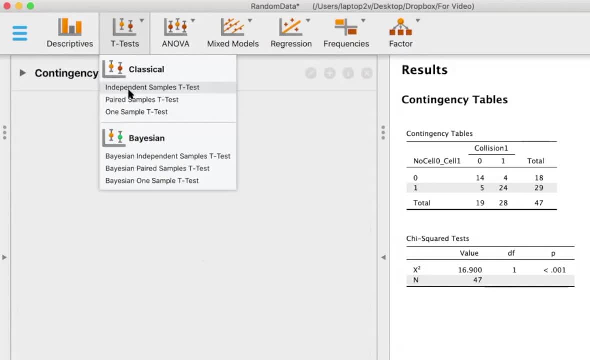 participants were in another condition. That contrasts with a within subjects experiment, where each participant was in both of your conditions, And so we don't have that. We've got two different groups of participants- one using their cell phones, the other not using their cell phones- in our different conditions. So that's why. 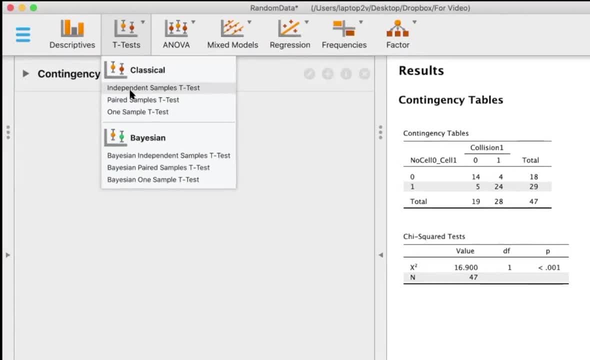 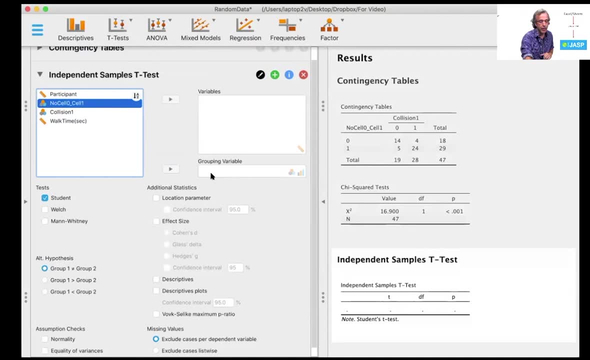 we need to use an independent samples t-test. So you select that And what you get is a little screen that asks you number one, your grouping variable. So that is a variable that are no cell versus cell that tells which group each participant's in. 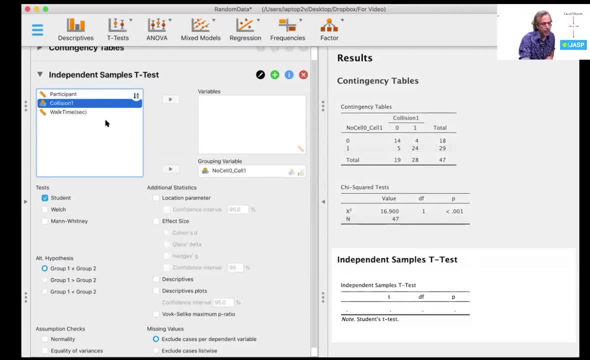 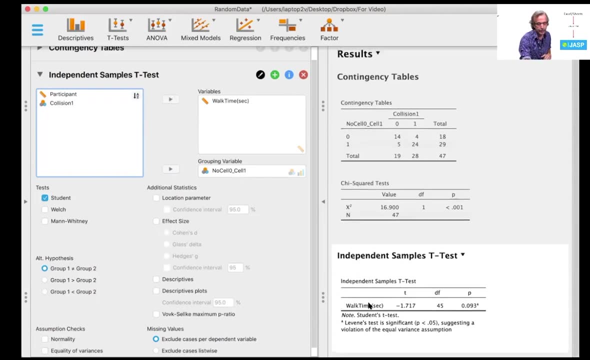 So let's put that down in grouping variables And then our variables here. this is basically our dependent variable, And let's put our walking time here. So that's our continuous measure of something, our continuous variable, And what we can see here is, it's done, the first part of our 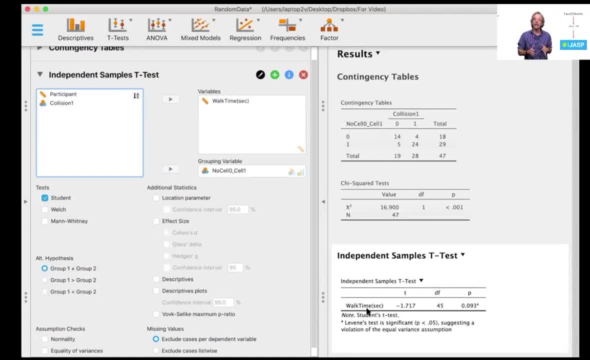 independent samples, t-test. When you do these, it's really nice. It's really nice also to print out your descriptive statistics. You want to know the mean scores in each of your conditions, So let's click descriptives right there, And then we're going to get below our 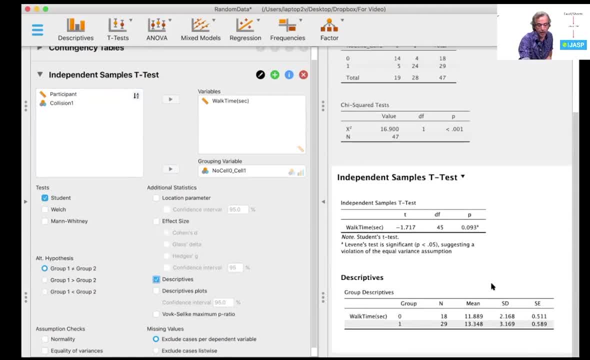 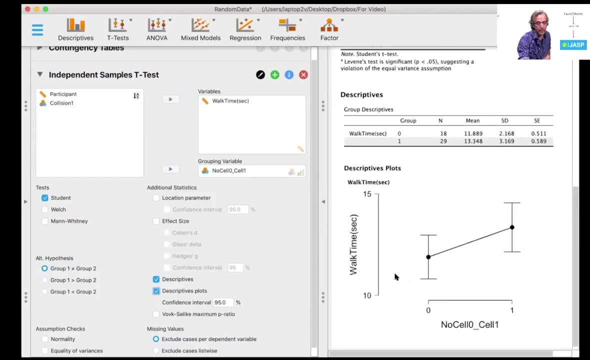 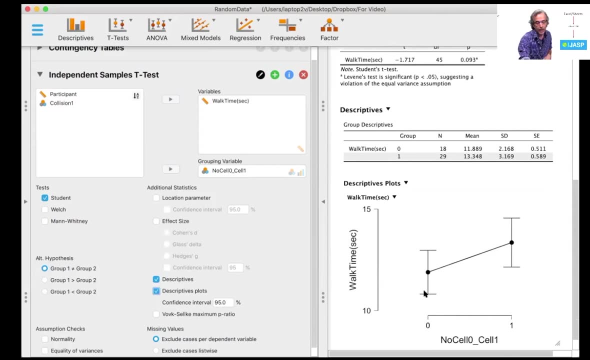 p values and t values, the means and standard deviation and also standard error, And if you want, you can even go ahead and do a plot. Takes a moment to do that- And there's our plot of our two averages. So what we're looking at here in the plot is: it looks like people are doing a lot of. 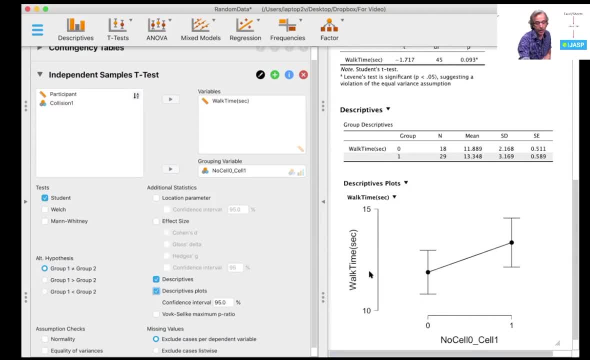 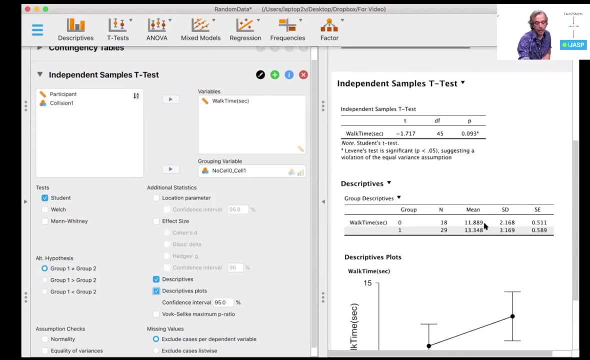 things. People are going maybe a little faster when they're not using their cell- a lower walking time- and a little slower when they're using their cell phone. That's reflected in the means here, So you can see we've got a 13-second mean among our participants who are using their cell phone. 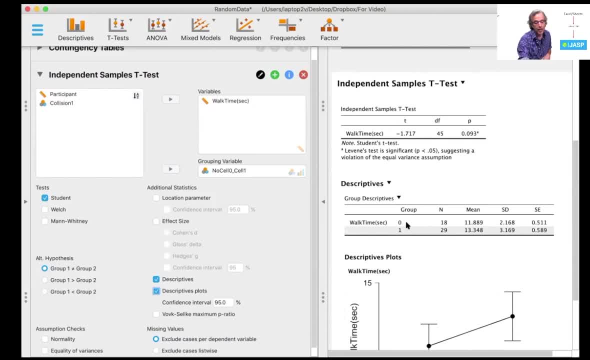 And then an 18-second or 11-second- mean sorry- in the participants who are not using their cell phone, And as we go up here, this is the results of the statistical test assessing the degree to which we can be competent. 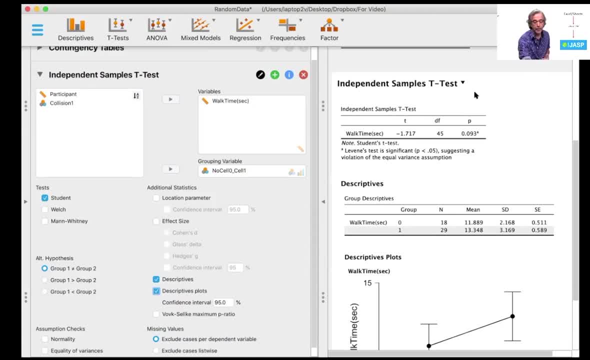 So we're going to go ahead and do a plot. And then we're going to go ahead and do a plot And, as you can see here, this p value is a little larger than the p value we had last time. It's 0.093.. And so that's going to be maybe a little too big for us to be confident that we've got. 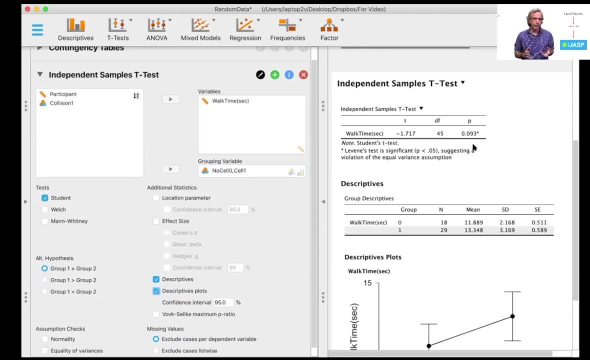 an effect. that's for real. So once again, what that p value tells you. maybe you can start repeating this after me. If you did the experiment over and over again and there were actually nothing there, this is going to be a little too big for us to be confident that we've got an effect. 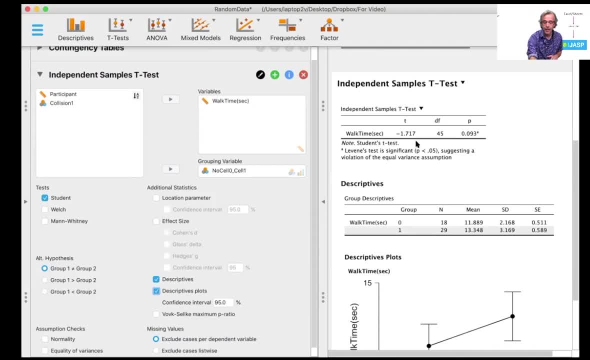 This is the probability that you'll get a test statistic, in this case the t value, and more or less a difference in means, as big as you saw it, of that size or bigger. And so what we're looking at here, to rephrase slightly- is the probability that, if you did this experiment over and over, 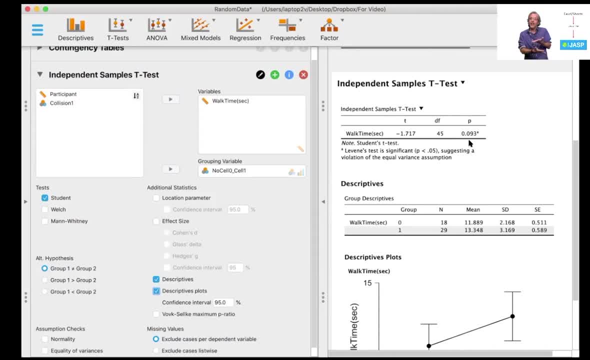 again. you'd observe an effect this big if, in fact, there were nothing there, And so again, we're looking for a nice small p value. Really, we want it to be below 0.05.. 0.01 is even better, And this p value is bigger than 0.05.. So we shouldn't be very confident. 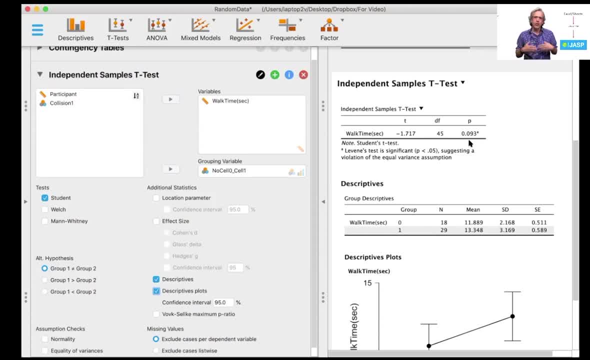 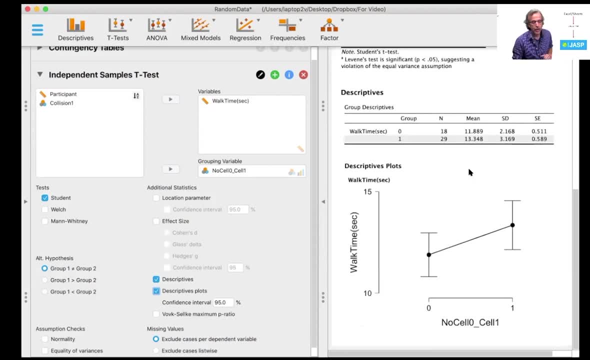 in this case, in the difference between our means. You would call this difference non-significant. Okay, So that's how you do: a test of the significance of a continuous variable and a test of the significance of a dichotomous variable. So as a reminder,